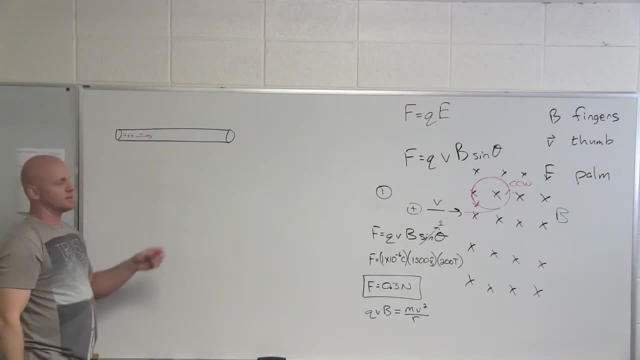 All right. so let's say I had a long cylinder, a long hollow cylinder, with positive charges flowing down the length of that cylinder. They were just flowing down the entire length of the cylinder. So let's say I applied a magnetic field and again I'm going to put, I'm going to apply. 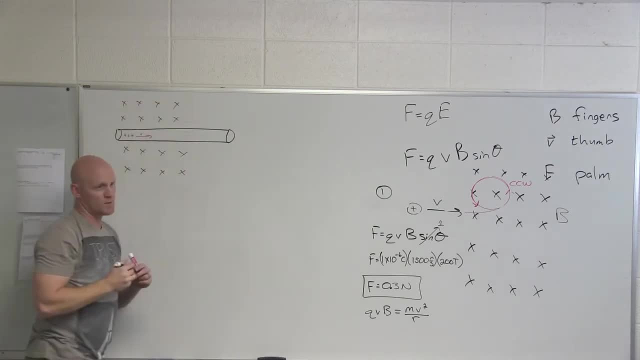 this magnetic field into the board everywhere where this lovely hollow cylinder is. My question is: so those charges inside this hollow cylinder, what direction is the force they feel? Cool, Same thing we did here earlier. It's going to be up just like it was initially here as well. 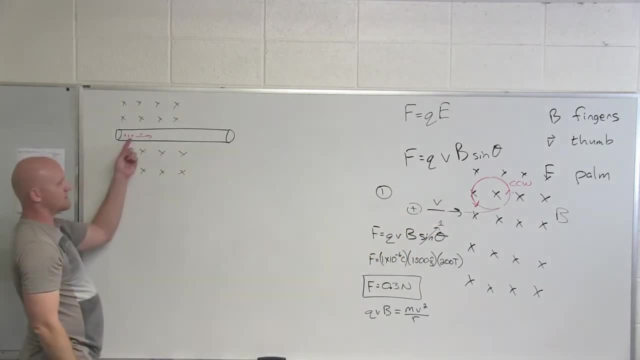 right. Nothing changed here. Well, technically, what I didn't tell you is that the positive charge is moving in here. That is actually. it's not a hollow cylinder, It is a metal wire, So and what we have flowing through it is current, conventional current, in this case the. 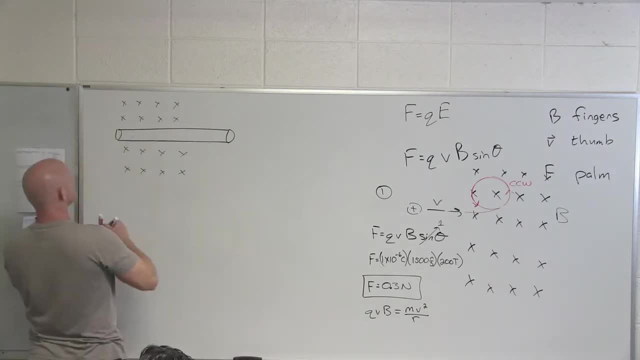 pretend flow of positive charges in our metal wire here, And so in this case we've got a current I flowing to the right through this wire and it's going to feel a net magnetic force upward, as we just demonstrated, exactly the same way, And we have another right-hand rule for 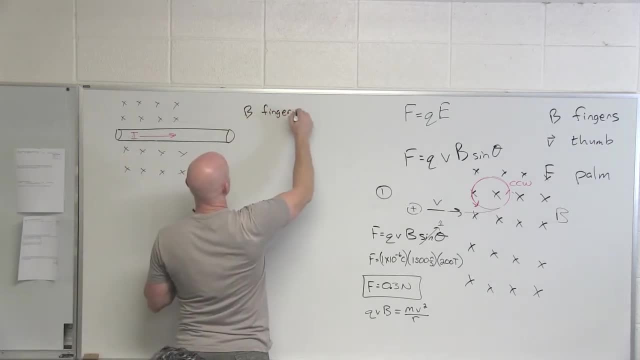 this. So your magnetic field is still your fingers, And guess what your velocity is now? or sorry, guess what your thumb is now, since it's not technically velocity, It's the direction of the current. but the current really is just the direction of the flow of positive charges. 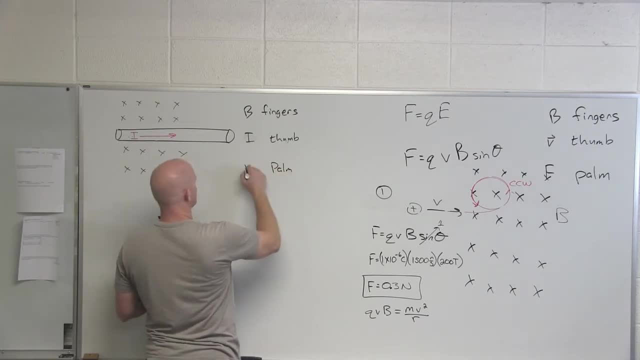 Cool. And then, coming out, your palm is still the force, And so technically this is a separate right-hand rule, but really it's kind of the same right-hand rule. Now let me ask you a question, though This is conventional current. 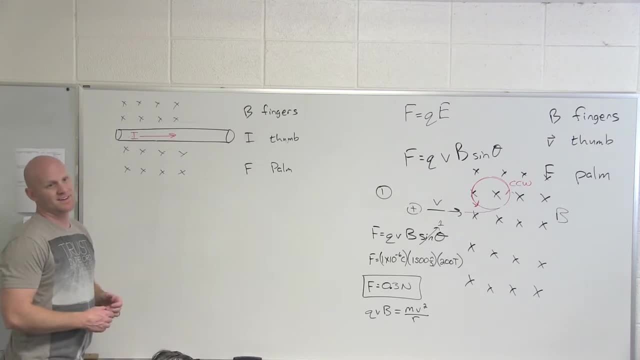 imaginary flow of positive charges. What's real? current Negative charges that are really flowing where The opposite direction. So let's take that into account. So magnetic field still points in, but now my negative charges are actually flowing this way, But because they're negative. my palm points down, but because they're negative. 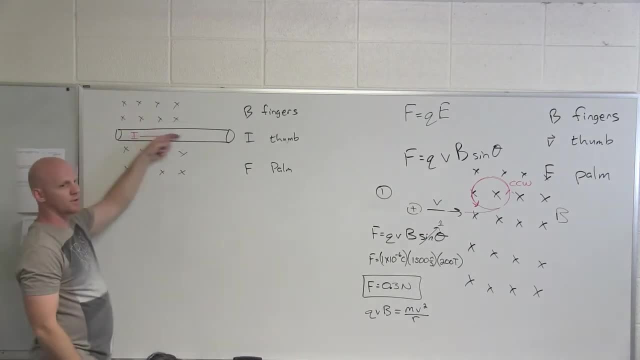 the force would still point up. So whether you look at it as conventional current flowing to the right or actual electrons flowing left, the force is the same either way. So you can't well again, for positive charges, the force comes out your palm, but for a negative charge, 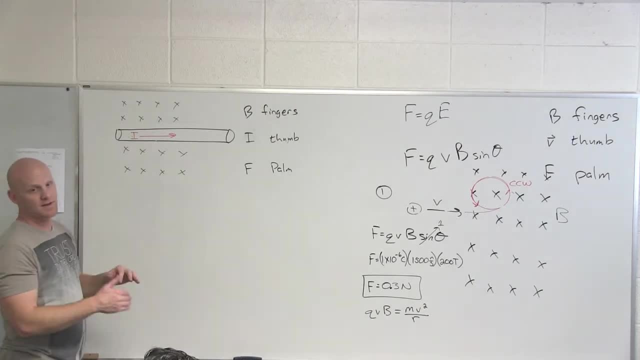 the force comes out the back of your hand. It's the opposite, Because whether it's conventional current positive charges flowing this way or it's electrons flowing the opposite way, So I actually can't tell the difference at the end of the day, real easy So, and it turns. 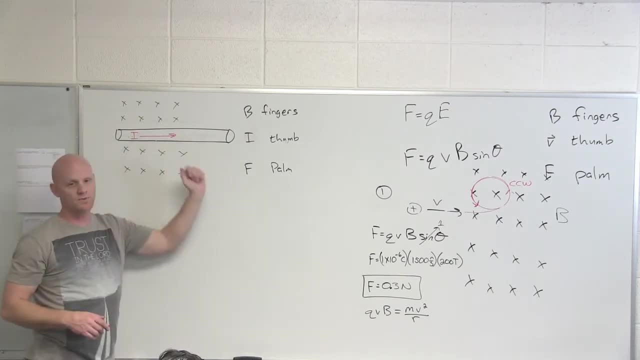 out. you know, back a couple hundred years ago they guessed wrong and they thought it was positive charges flowing this way. but through a wire it's actually negative charges flowing this way. But we can use our right-hand rule and figure out: the force would be up regardless of. 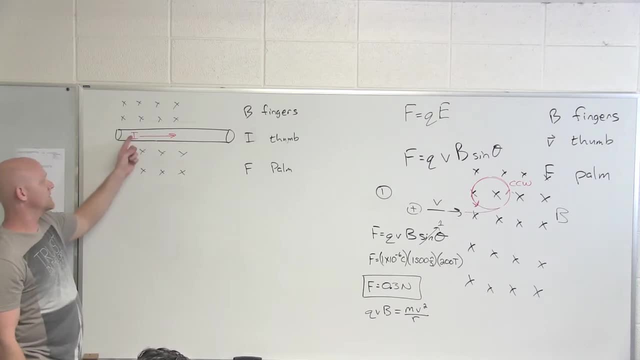 how you took it. Cool, but be careful When you see the letter I here. we're giving you conventional current, not the actual flow of electrons, but conventional current. Okay, and it turns out that force proportional to the magnetic field. so and the current and the length of your wire. 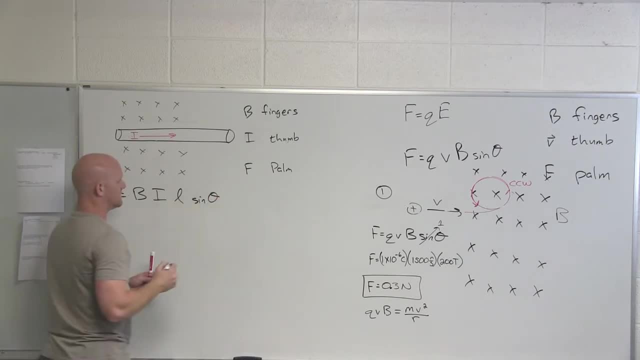 and again, there's actually a cross product in this and you have a sine theta. And so in this case, if your current and your magnetic field so aren't exactly 90 degrees apart, then you'll have to factor in that angle theta. In this case, how far apart is the magnetic field and the? 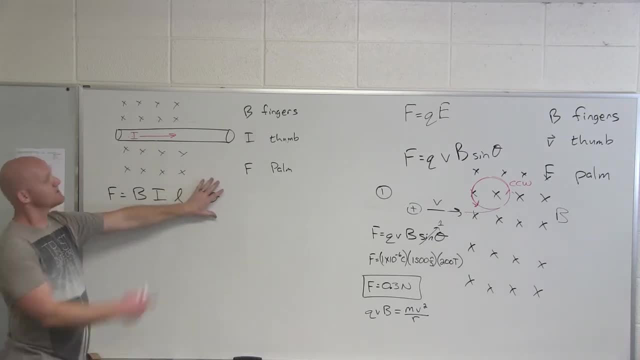 current They're 90 degrees apart, So you have to factor in that angle theta. So you have to factor in that direction. So 90 degrees apart, and sine of 90 is 1.. It's going to go away for. 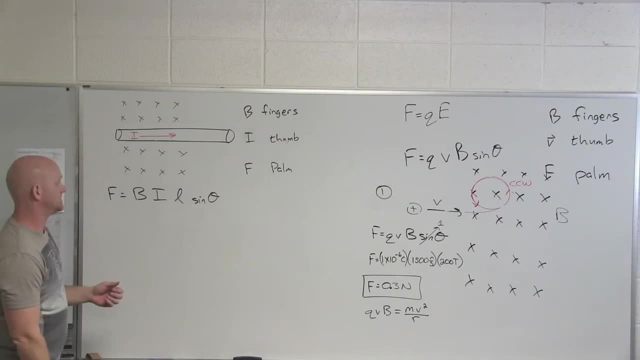 this example, stuff like this, But cool just now, the force on a current carrying wire. Yeah, That wire's feeling a net pull upward. So often times we'll see a question like this and you'll find out that this wire is hovering in the air. And if it's hovering in the air, 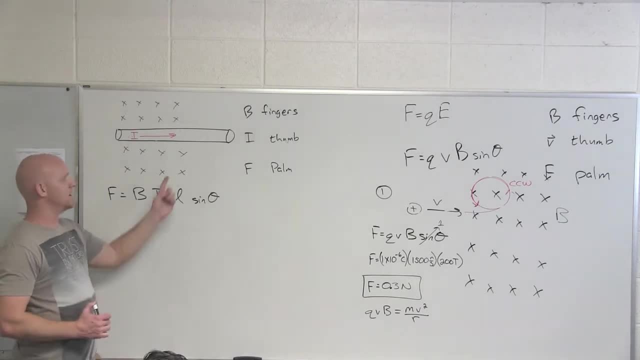 what must be true, Same, I mean, the upward force must be perfectly balancing A Downward force. And what downward force would we be talking about? Gravity, And so we'd find out that this guy equals mg. They're an equal magnitude, opposite directions. 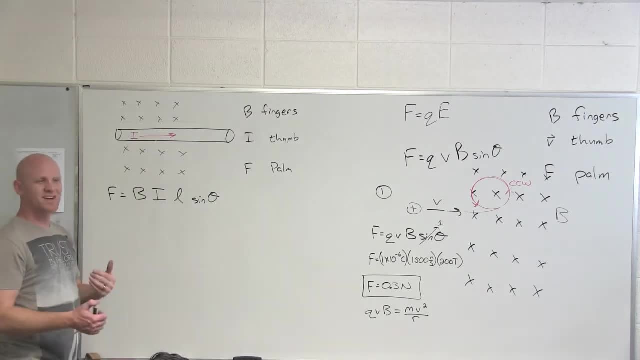 Cool, And you can find the mass. or you can find the strength of the magnetic field, if you knew the mass, or vice versa. Essentially, they'll give you all the variables except one, Cool. So let's look at question number two. 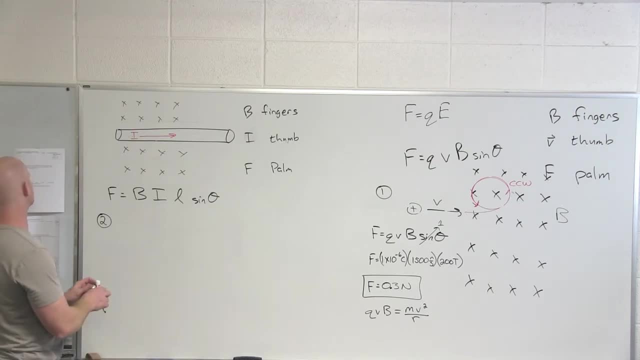 Question number two says a wire with 10 amps of current, so directed west horizontally. So in this case We'll call this west. Ah, With a linear mass density- this is going to be fun- of 0.5 grams per centimeter. 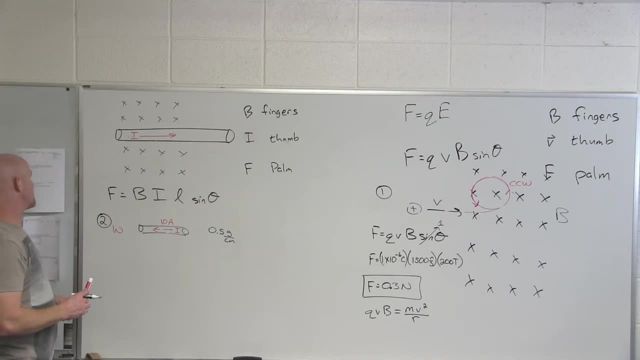 It's suspended vertically in the air due to the presence of a magnetic field, Exactly what we were just talking about. So what is the magnitude and direction of the magnetic field? So in this case, if we set up our free body diagram on this thing, we've got an upward force. 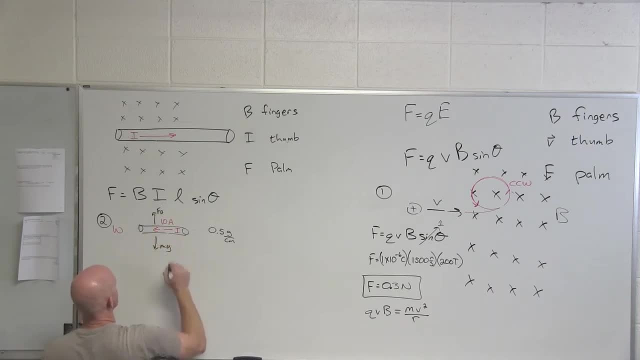 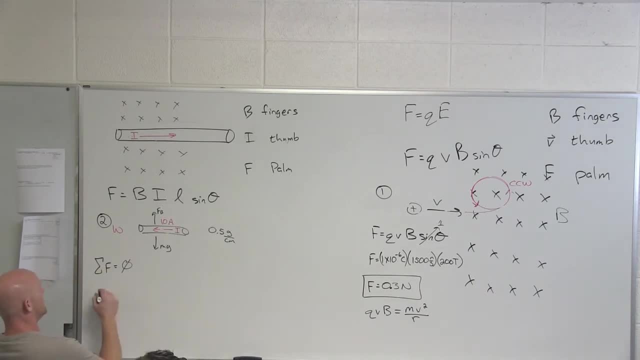 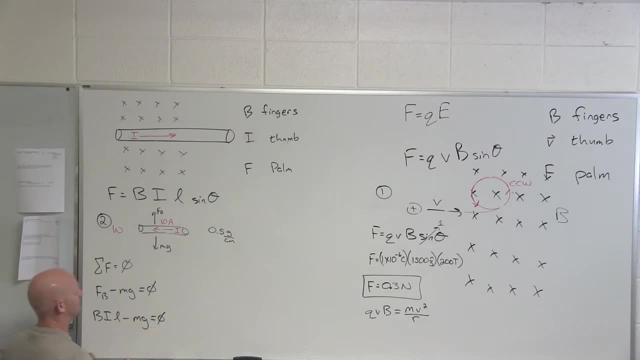 since they're perpendicular, Cool. What are we solving for in this case? Magnetic field, Magnetic field. So if we do some rearranging here, So your magnetic field is going to equal m g over i l. So do we know the mass of this wire? 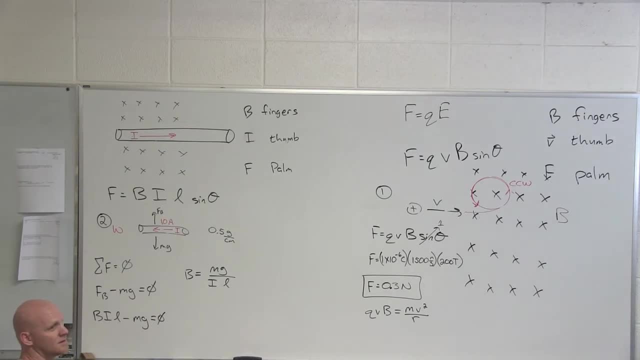 No. Do we know how long it is? No, No, What do we know in regards to that? We know the mass per unit length is this: 0.5 grams per centimeter. So we know that m over l is 0.5 grams per centimeter. 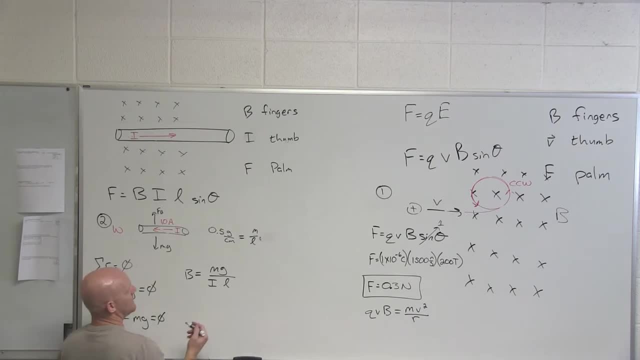 So in this case we know m over l as a whole. Now do I want it in grams per centimeter? What units do I want it in? Kilograms per meter. Kilograms per meter. So how do I get this in kilograms per meter?